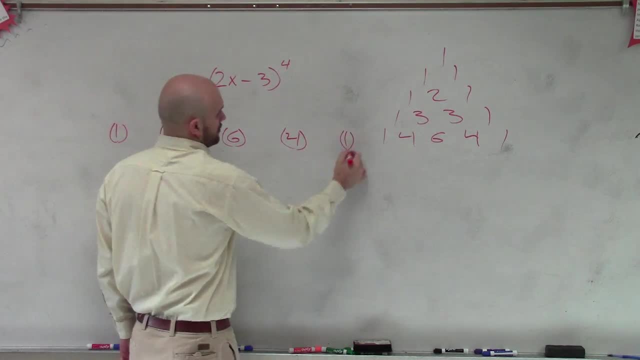 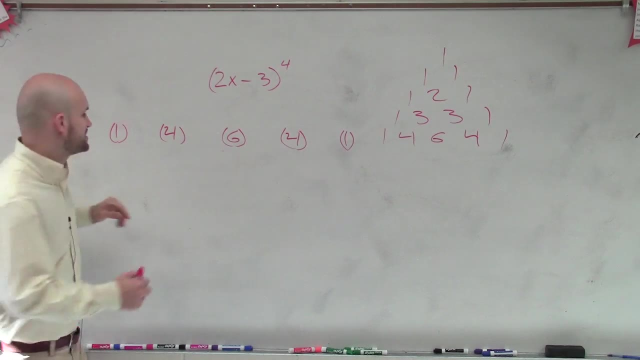 All right, Then we know that on my first term- remember- we've got to keep that to its 4th power. So this one's going to be 2x to the 4th Right, Then it's going to be 2x cubed. 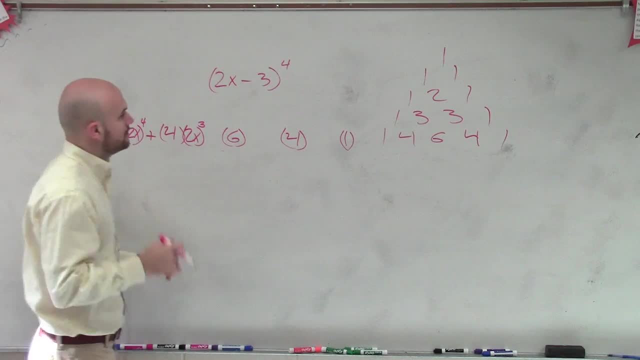 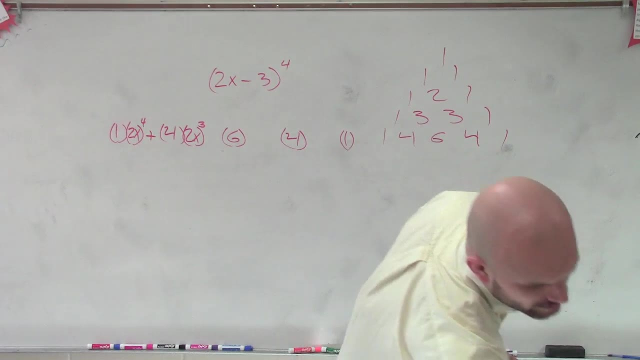 1, 2,, 3, 4.. Sorry, Yeah, I haven't Let me actually write this a little bit farther. So we have 1, which we don't really care about because the 1's not going to change. 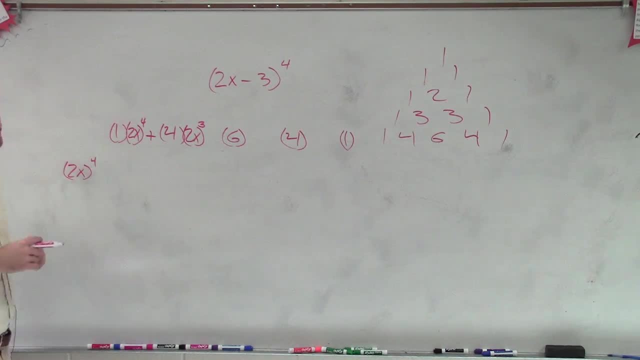 So I have 2x to the 4th, Yes, Okay, Then I multiply by 4 times. it goes now to 2x cubed, Right, But then, remember, now it's cubed, so now I have my negative 3.. Right, So now I have negative 3 raised to the, which is 1st power. Right, Because, remember, it starts at 0, then goes to the 1st power. 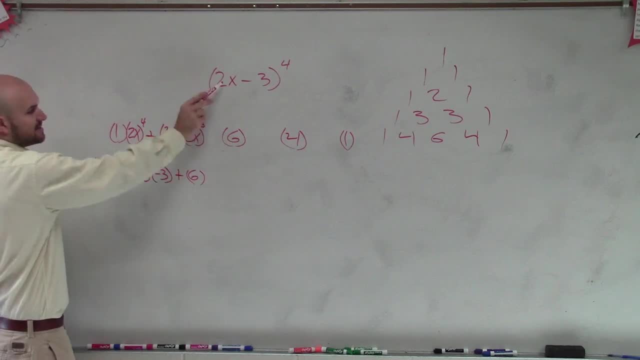 Plus 6 times. now it's 2x raised to the 2nd power Right. This 2x starts at 4.. Then goes to 3.. Then goes to 2.. Then goes to the 1. Right. 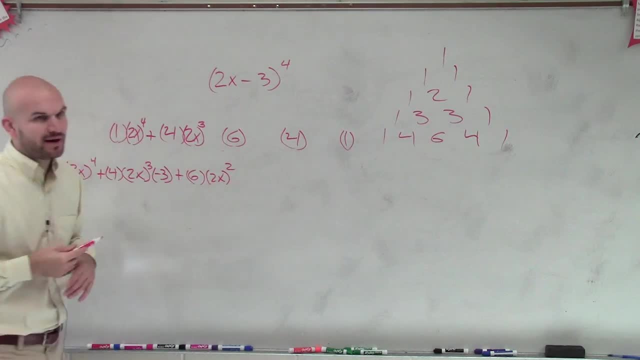 The only difference is- now I have different coefficients- that I'm multiplying it by Then. so let's go 2x squared and then my negative 3 gets raised to the what power 2nd power. So it's negative 3.. Now it's negative 3 to the 2nd power. 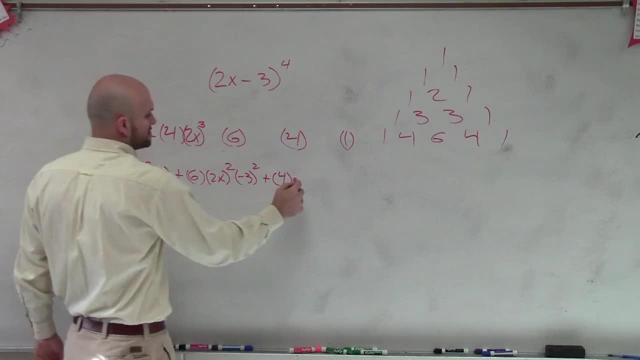 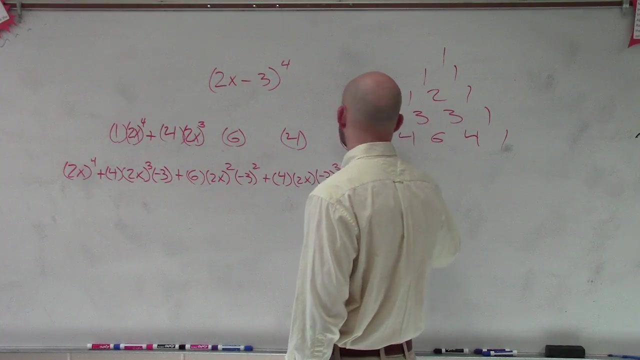 Then plus 4 times a, 2x to the 1st times negative, 3 cubed Right, And then plus that's 2x to the 0 times 1 to the negative, 3 to the 4th. 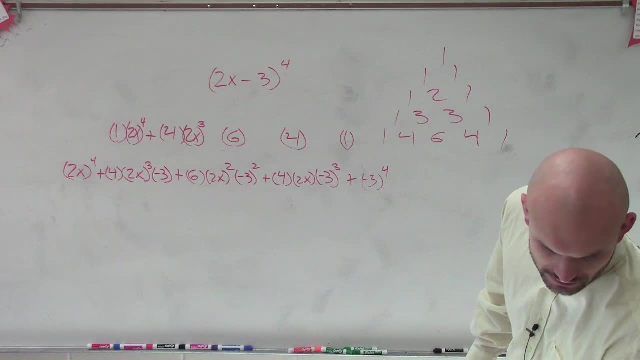 And then you can go ahead and multiply that out. So 2 to the 4th power, 2 to the 3rd power is going to be 8.. So 2 to the 4th power is going to be 16x to the 4th. 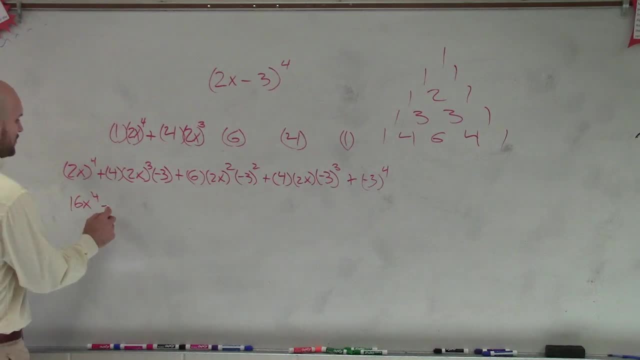 This is going to be a negative 12.. So it would be a negative 24.. Oh, I'm sorry, That's 8.. That's 2 cubed, That's 8.. 8 times 4 is going to be 32.. 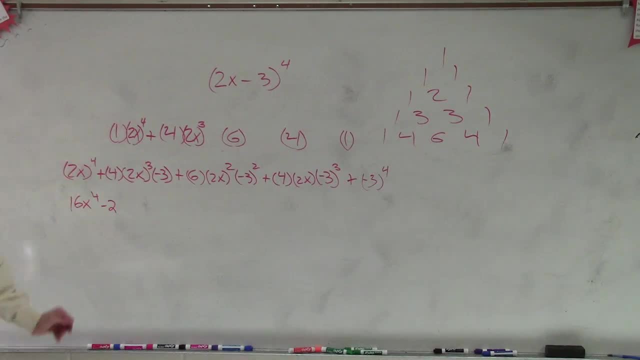 Times a negative. 3 is going to be a negative 60.. 32 times 3,, which would be a negative. What am I doing, Kelly? you have this, So we have 4.. So we have 8.. 8 times 4 is 32.. 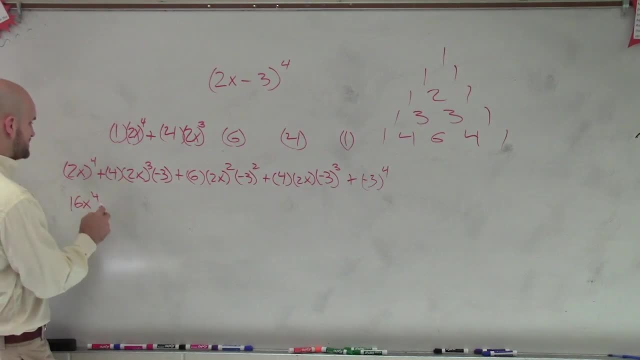 Times a negative 3,, which would be a negative 64,, which would be a negative 96.. That's x cubed, And then we have plus 6.. So 2 squared is going to be 4.. 4 times 6 is 24.. 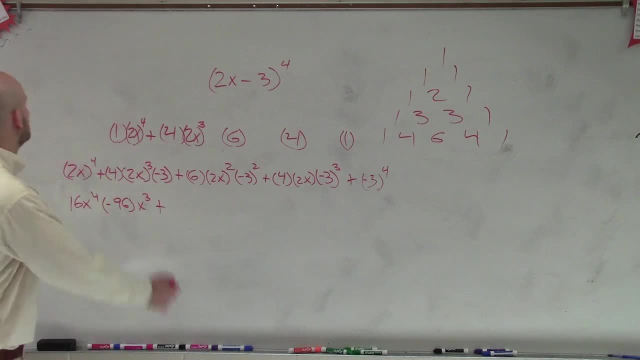 And then 24 times 9 is- I don't know- 216x squared. Then here I have negative 3.. Can somebody do 27 times 4 times 2, please, A negative 27, actually. So it's a negative 216x. 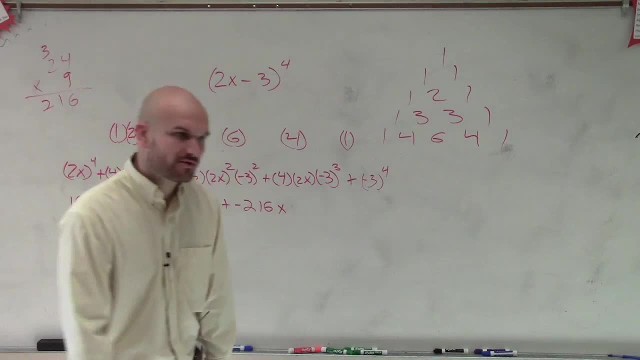 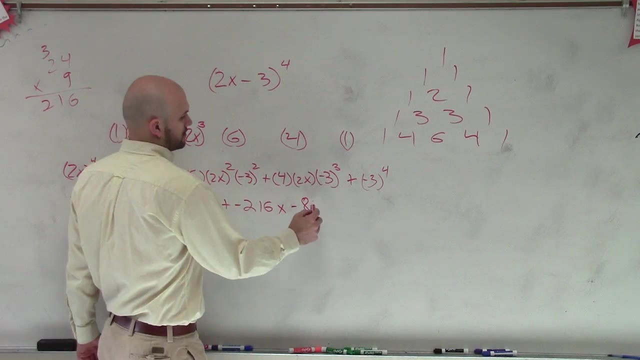 All right, And then this one negative 3 to the 4th power is Negative 81.. 481.. 481.. What was that, Kevin? Negative 3 to the 4th is 481.. Yeah, it's positive 481.. 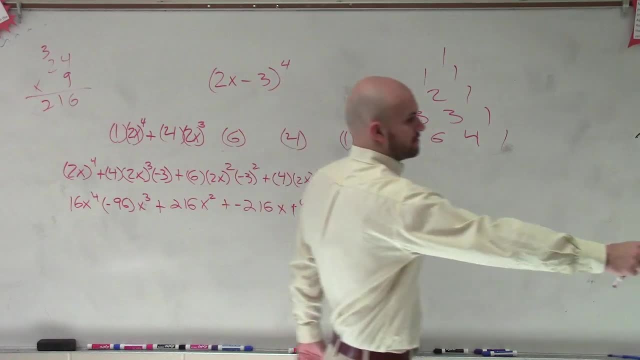 How is it 481?? I got 81.. Two more weeks, it's like Leg in two more weeks. I'm sorry It's negative 481.. I don't know, That's what you guys told me. I said 81.. 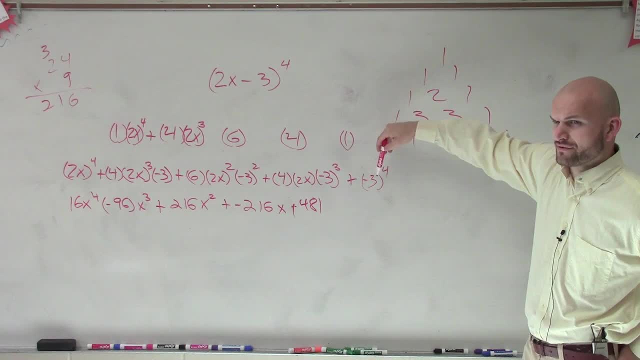 Okay, but it's. It's negative 81.. Negative 81.. You have to put parentheses: Negative 3.. It's going to be positive, It has to be positive. So 3 times 3 is 9.. Times 3 is 27.. 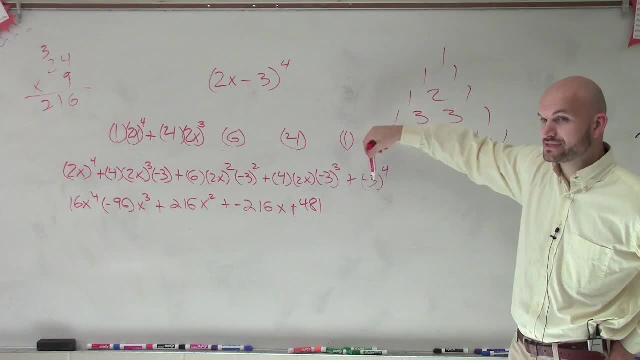